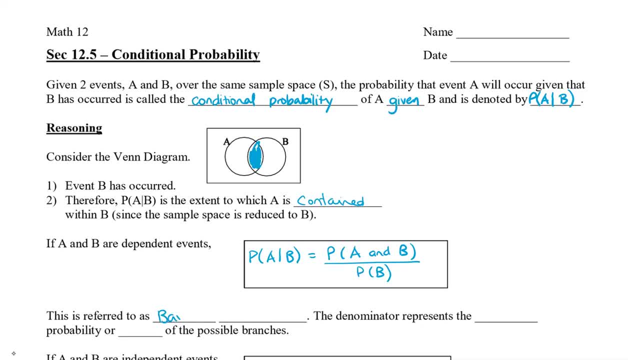 Now this is referred to as Bayes formula by a mathematician named Thomas Bayes. So the denominator represents the total probability or the sum of all the possible branches. if we drew a probability tree. Now, if the two events A and B are independent, 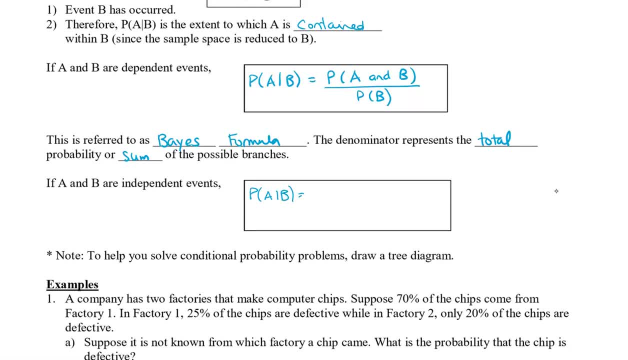 then we have the probability of A, given B is equal to the probability of A times the probability of B, because probability of A and B are independent And this would all divide by the probability of B. However, now the probability of B will cross off in the numerator and the denominator. 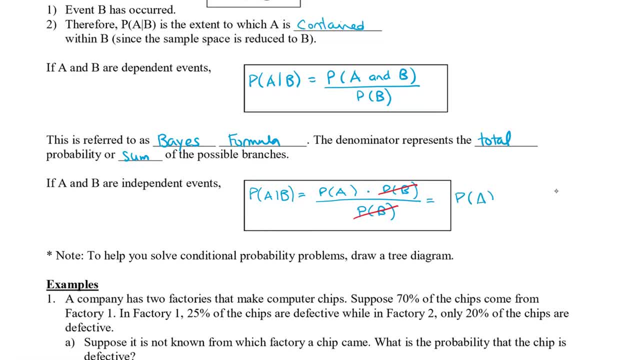 so then we're only left with the probability of A, And that's because if they're independent, that means that one does not depend on the other. So it doesn't matter if B has happened, P of A or the probability of A will still occur. 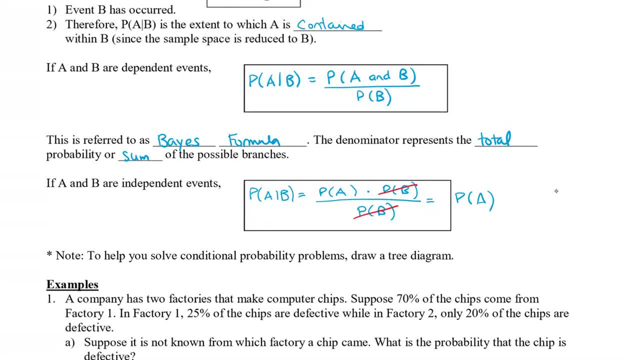 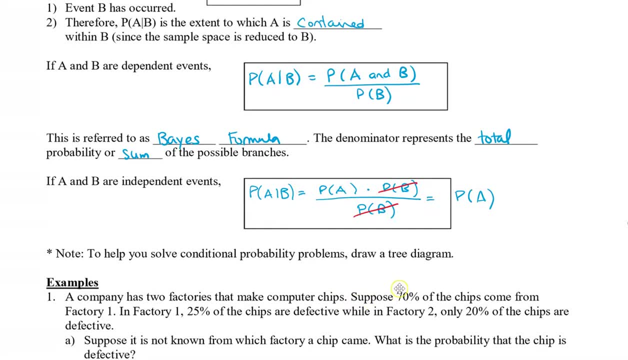 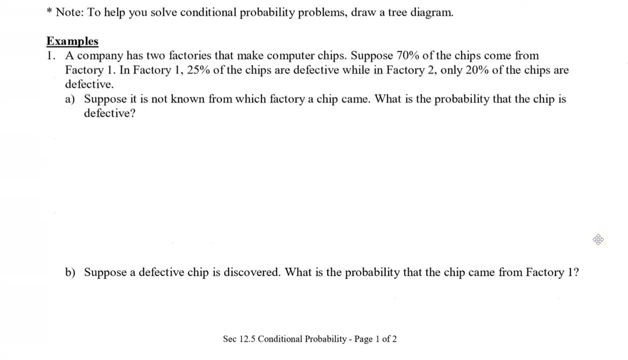 Now, to help you solve conditional probability problems, I recommend that you draw a tree diagram so that we can take a look at all the different branches. Let's take a look at an example to illustrate this. A company has two factories that make computer chips. 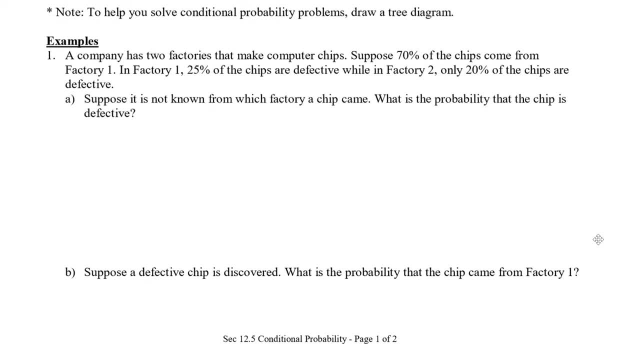 Suppose 70% of the chips come from factory 1.. So I'm going to draw a tree to represent this. So we have factory 1 and factory 2.. So 70% come from factory 1, and 30% come from factory 2.. 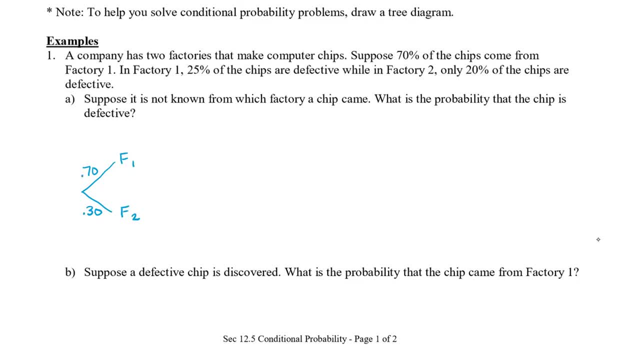 Or 0.7 and 0.3.. So in factory 1, 25% of the chips are defective. So we're going to branch out from factory 1.. So those are defective. I'll call it D and that would be 0.25.. 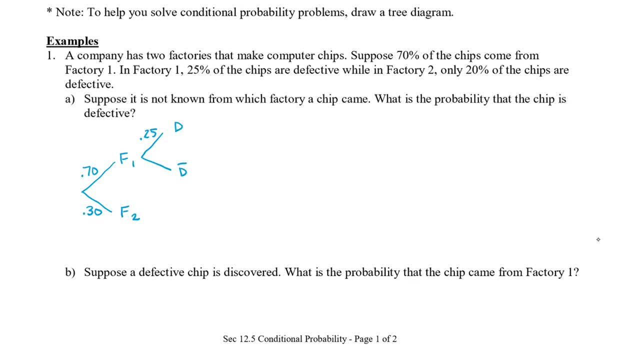 And those are not defective, I'll put D with the line at the top and put 0.75.. While in factory 2, only 20% of the chips are defective. So D and D with the line, the complement. 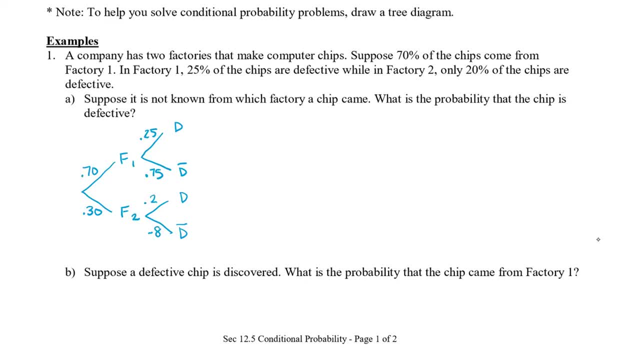 So you have 0.2 and 0.8.. Now suppose it is not known from which factory a chip came from. So the question is: what is the probability that the chip is defective? So we can say that the probability that the chip is defective. 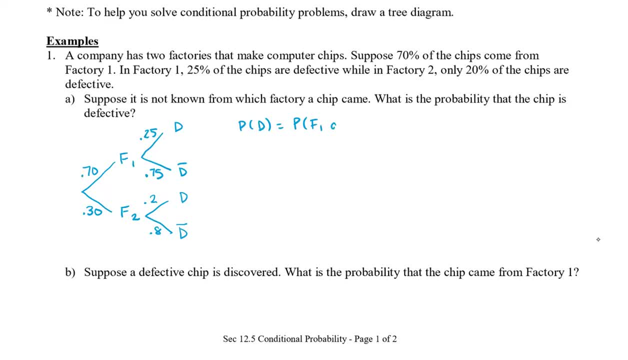 is equal to the probability that it is from factory 1 and it's defective. Or we can say that it's the probability of factory 2, or it came from factory 2 and it's defective. Now, if we write this out formally, 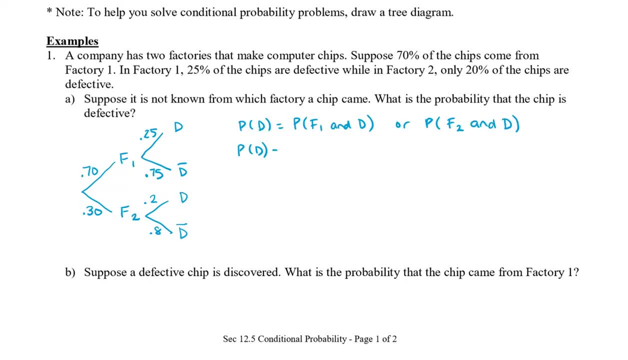 this is what it would look like. The probability that it's defective is equal to the probability that it's from factory 1 times the probability that it's defective, given that it's from factory 1, plus the probability that it's from factory 2. 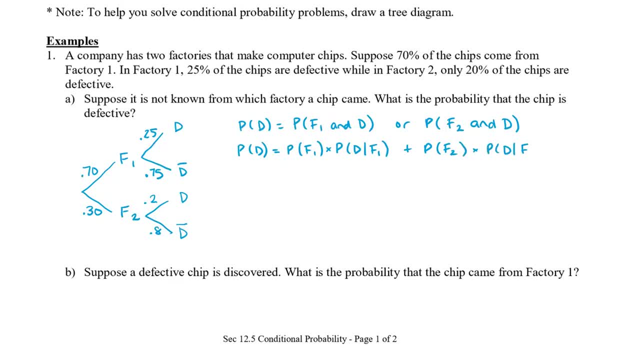 times the probability that it's defective, given that it's from factory 2.. Now that's kind of really a bit long-winded, But really what it means in terms of the numbers is that the probability that it's from factory 1 is going to be 0.7. 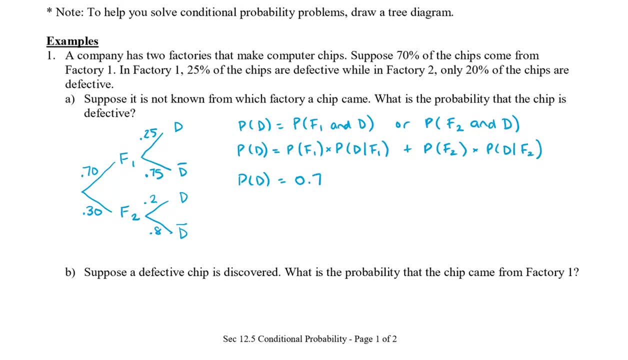 and the probability that it's defective, given that it's from factory 1, will be 0.25.. That means that we have to follow the branch from factory 1.. So that's 0.25, and then in factory 2, so the probability that it's from factory 2 is 0.3. 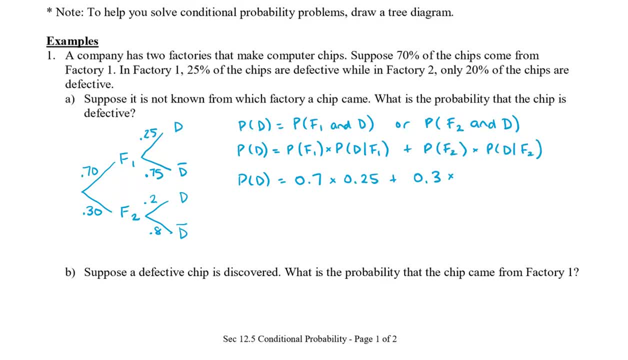 and then times the probability that it's defective. given that it's from factory 2, means that we follow the factory 2 branch. So that would be 0.2.. So typing everything into our calculator, we get 0.235.. Now let's take a look at a question. 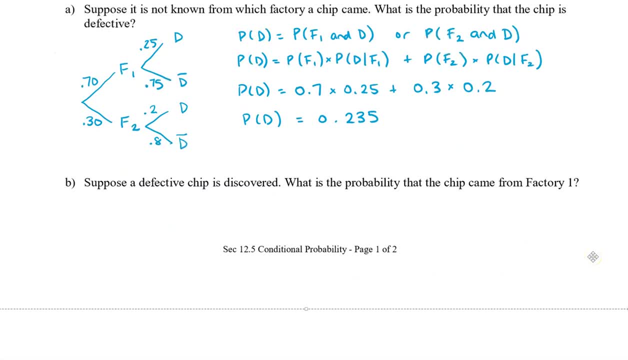 that involves conditional probability. Suppose that a defective chip is discovered. That also means if a defective chip is discovered or given a defective chip is discovered, what is the probability that the chip came from factory 1? So we want to find the probability that the chip is from factory 1. 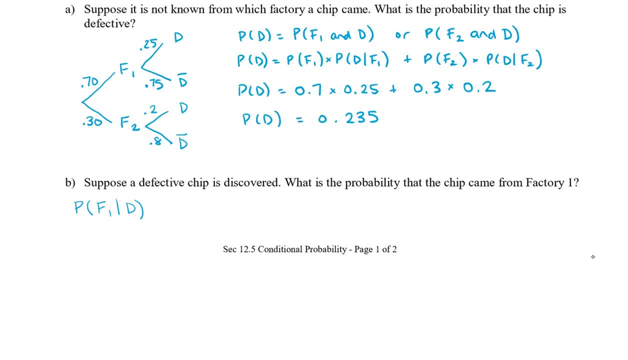 given that it's defective. Now, we know that it's in this order because the question says: what is the probability that the chip came from factory 1? And that is what we write first. So the probability that it came from factory 1, given that it's defective. 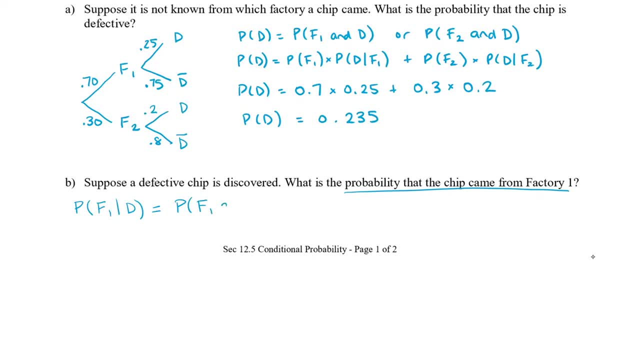 is equal to the probability that it's from factory 1 and defective divided by the probability that it's defective. So this is equal to so if it's from factory 1 and it's defective, that means it's going to be 0.7. 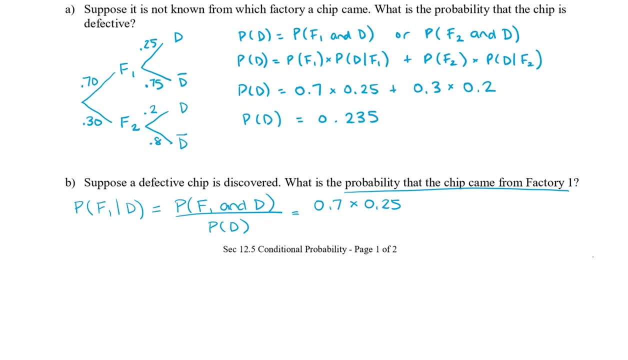 times 0.25, and if you look above, that's this part here, And then we divide by the probability that it's defective. So a defective chip, remember, can come from factory 1 and factory 2.. So we're going to use this number: 0.235. 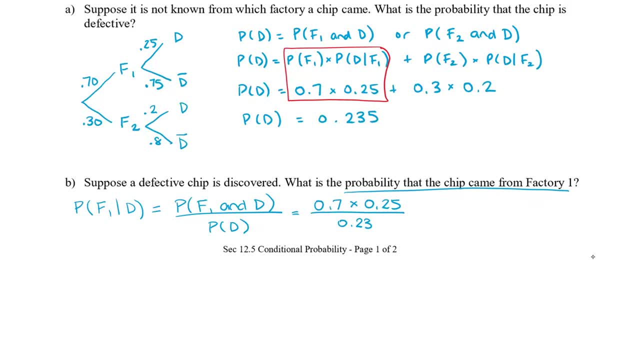 as our probability of being defective. So we multiply this out, we get 0.175 divided by 0.235, and then when we divide, we get 0.7447, which seems a little bit high but it's not because remember most of the chips. 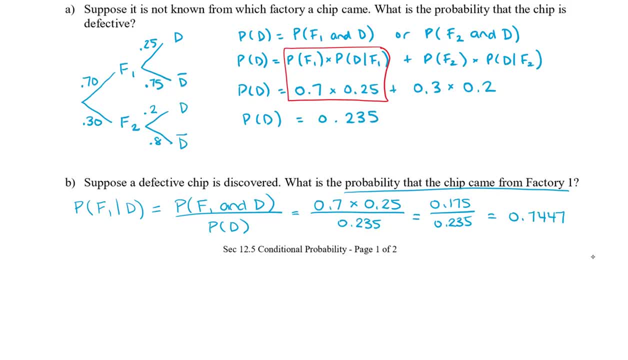 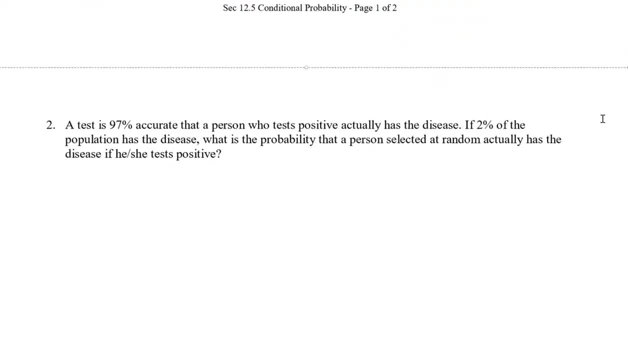 come from factory 1, and then there are more defective chips from factory 1 than there are from factory 2.. Let's take a look at another problem. So this is quite a common one that you'll see quite often A test is 97% accurate. 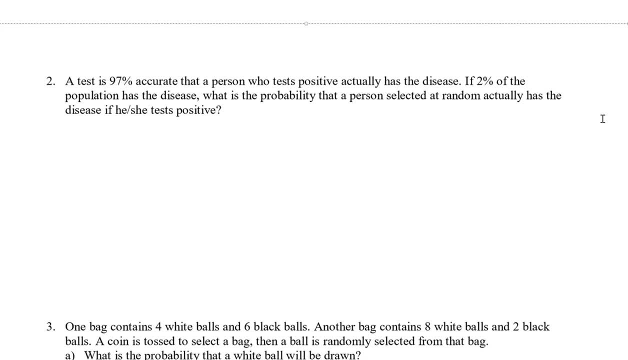 that a person who tests positive actually has the disease? If 2% of the population has the disease, what is the probability that a person selected at random actually has the disease if he or she tested positive? Alright, we're going to start with a little let statement. 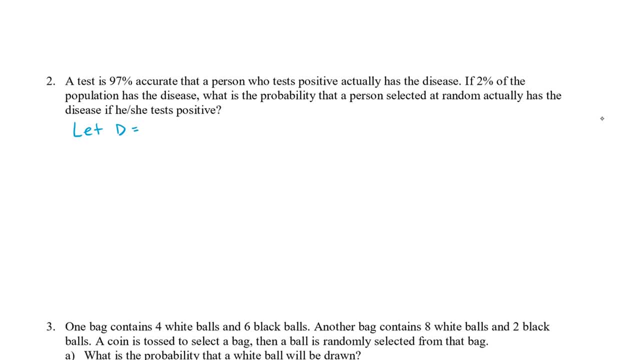 so that we know what everything stands for. So we're going to say d equals has the disease, and then we're going to let t equals test positive, because it actually says here what is probably selected at random actually has the disease if he or she tests positive. 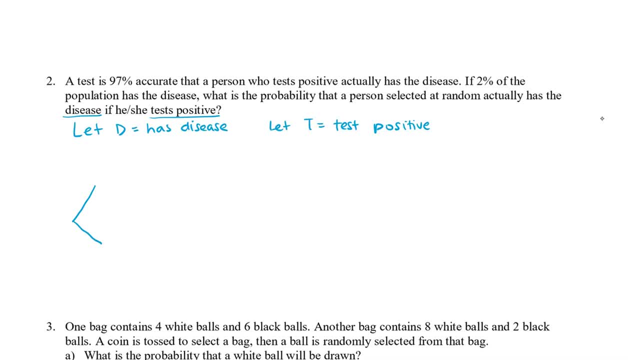 So we're going to draw our tree, starting with our population, so d, and then d with a line on the top, So 2% have the disease, so 0.02 and then therefore 0.98 do not have the disease. Alright, now we're going to talk about 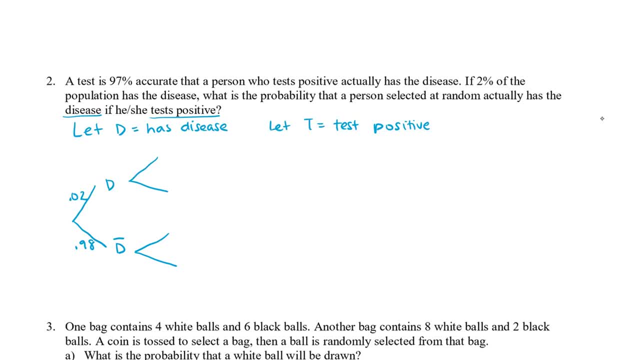 the testing part. So we have test positive and does not test positive. So if the person has the disease, they should test positive 0.97 or 97% of the time. If they don't test positive or they test negative, that would be 0.03. 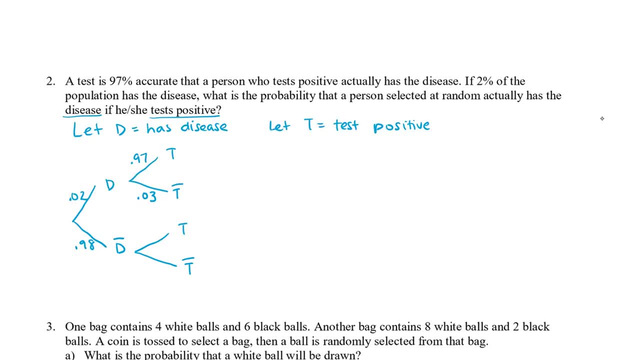 Now this is a little bit tricky, but if they don't have the disease, then the probability then that they don't test positive, that should be accurate, because the 97% is referring to the accuracy of the test. So if they don't have the disease, 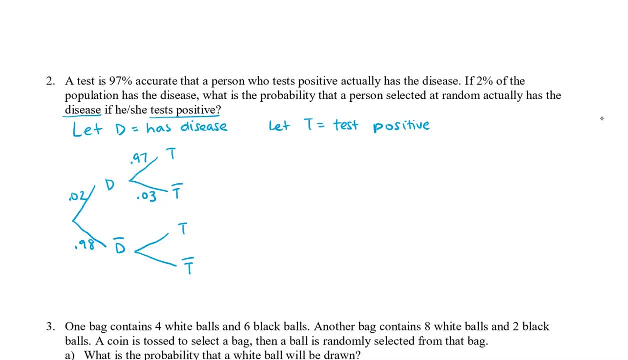 then they should be testing negative. So then, therefore, the 0.97 actually goes on testing negative because they don't have the disease. So therefore, testing positive would be 0.03, which is actually inaccurate because they actually don't have the disease. 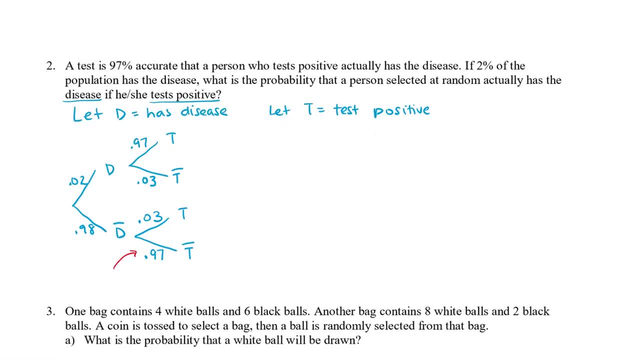 So let's write a little note about that in case we forget. So if a person does not have the disease, the person should test negative accurately. Alright, let's go back to the question. So what is the probability that a person selected at random actually has the disease? 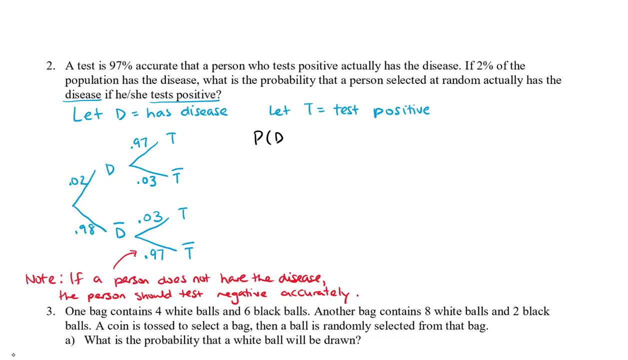 So probability of having the disease if he, she or test positive, given they test positive. So that equals the probability of having the disease and testing positive divided by the probability of testing positive. So the probability of having the disease and testing positive is 0.02. 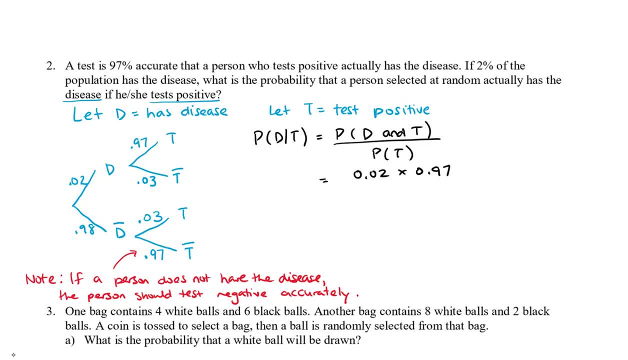 times 0.97, which is this branch over here, And that's divided by the probability of testing positive. Now there are two ways to do that. So one way is the 0.02 times 0.97, which is having the disease and then testing positive. 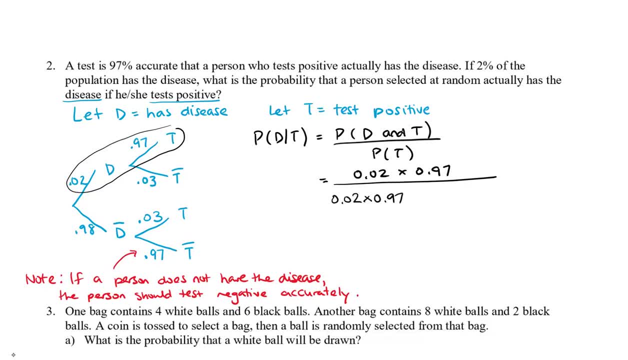 or we can not have the disease, so or so we're going to add not have the disease, which is 0.98, and then we're going to multiply that by 0.03, because they still tested positive, even though that is not accurate. 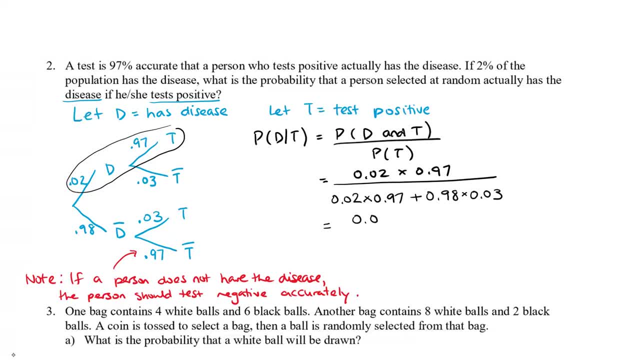 So in the numerator we get 0.0194, in the denominator we get 0.0488. but you can type all of this out together at one time- 0.398, and that's how you do a conditional probability problem. 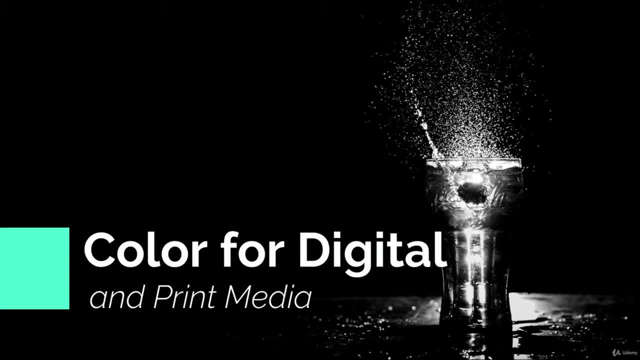 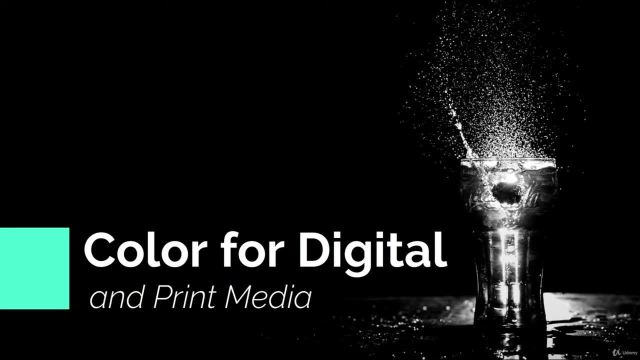 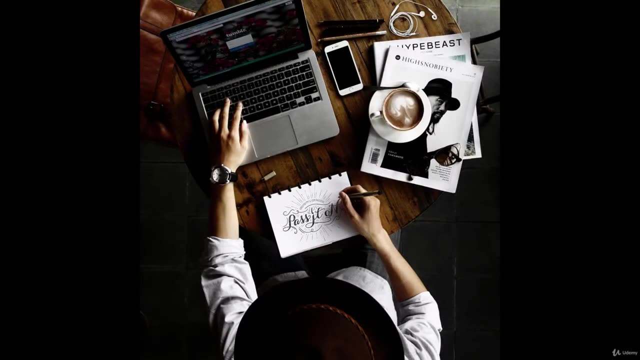 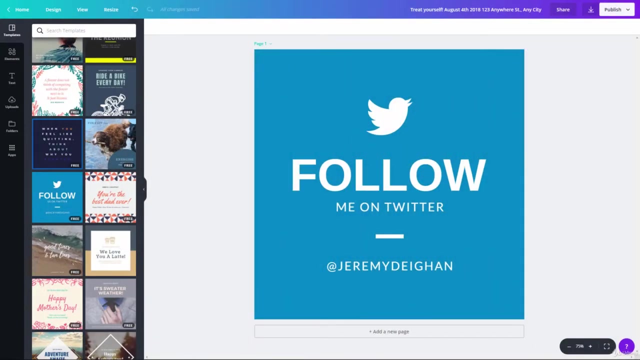 In this lesson, we will go over how you can use color, whether you are designing for digital media or for print media. Though they are pretty similar, they do have some differences that I would like to show you. First, let's take a look at using color in a digital medium. 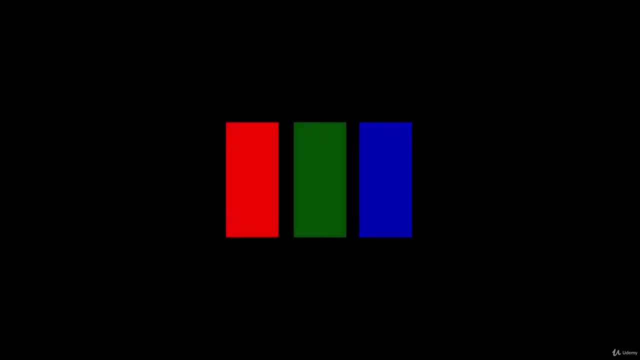 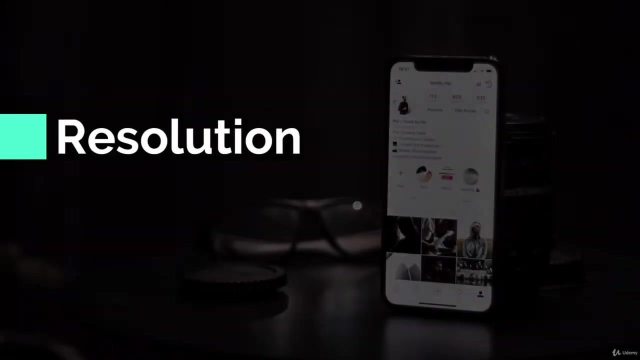 As you know by now, color is created on a computer by showing different amounts of red, green and blue lights that trick your mind into seeing all of the available colors. These lights combine together and are referred to as pixels. We can label the resolution of. 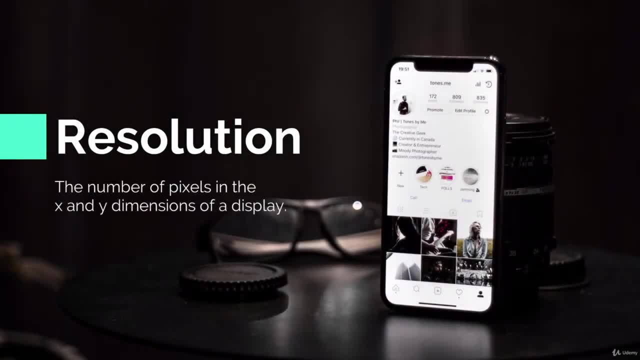 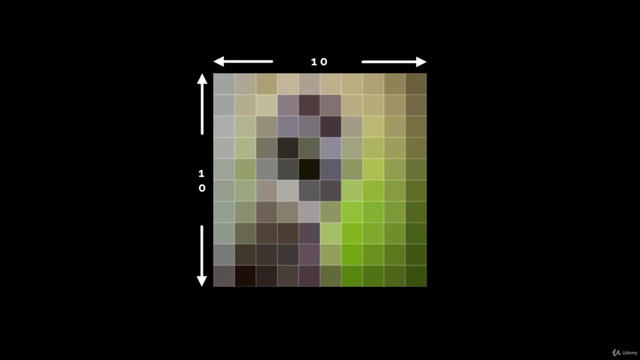 a screen or monitor by its pixel dimensions. So, for instance, imagine you had a very small device of only 10 pixels wide and 10 pixels tall. We would call the pixel size the pixel size of the screen. We would call the pixel dimensions 10x10 and there would be a total of 100 pixels.